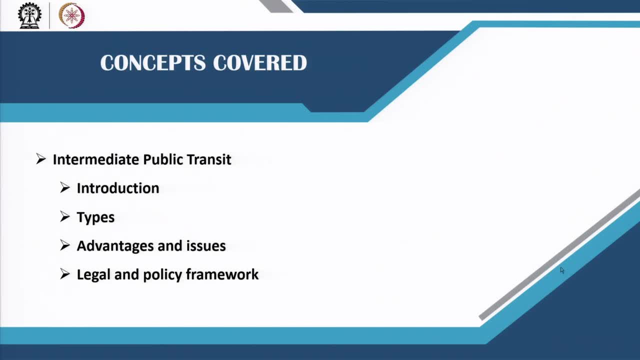 types of them. When can intermediate public transit or IPT, be advantages and when they- but as opposed to when they can harm the public transportation system? we will be looking at that and also giving you a overview of the legal and policy frameworks under which the IPT works. 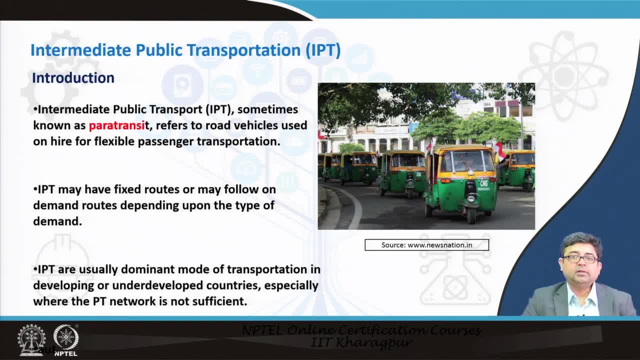 So when we talk about intermediate public transport, what we are trying to say is we are talking about those types of services that connect you to the larger public transport system in your city. right, So they can also be called para transit, but essentially those are the auto rickshaws. 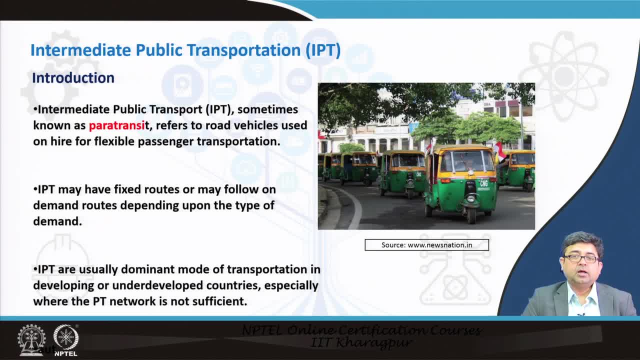 the cycle rickshaws or even sometimes taxis or després, or van pools or car pools that will take you from your origin to your larger public transportation network in your city right are meant as a bridge to connect you to the larger public transportation system in your 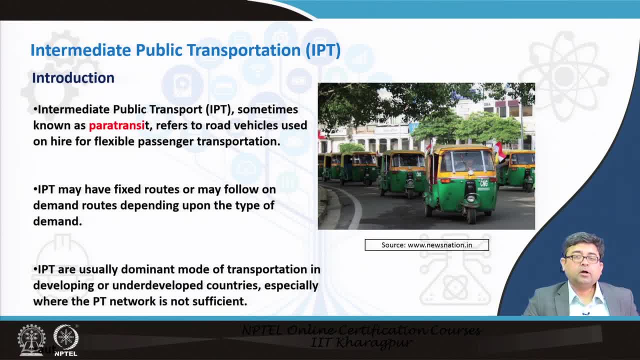 city. However, we have also seen, especially in the Indian context, that when a urban area does not have a public transportation system, or where public transportation system is not viable because of several reasons, IPT usually is the only public transportation system that is available in your urban area. right, 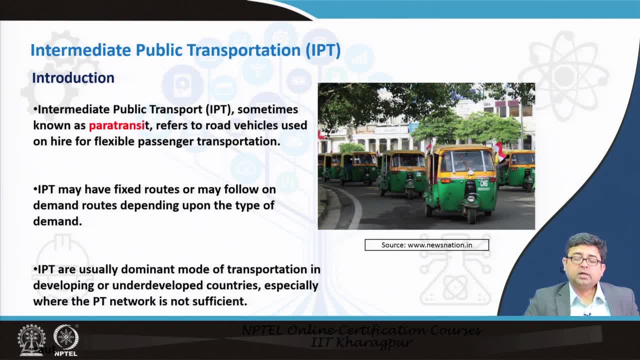 You may have come across shared auto rickshaw systems in many of the towns and smaller cities that you may have visited, where they almost act like a mini bus, where there are different people sharing the same auto rickshaw and are going to different destinations along. 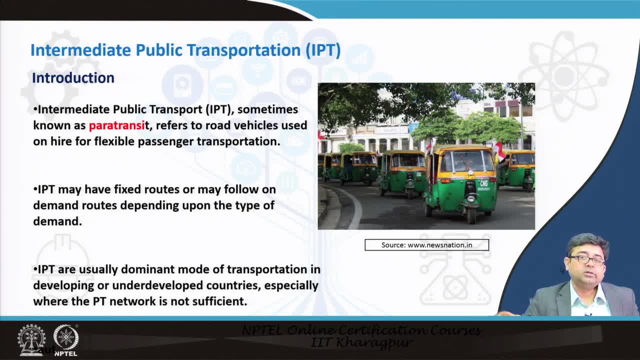 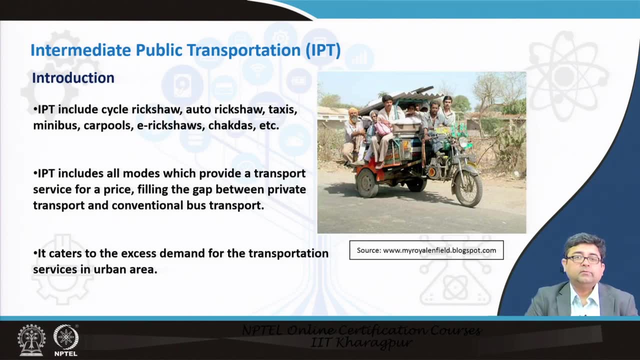 a fixed route. So we will look at how these different forms of IPT work, and are they, when are they beneficial and when are they not so beneficial for the city? ok, So when we say IPT, we include everything that provides you access to the public transportation. 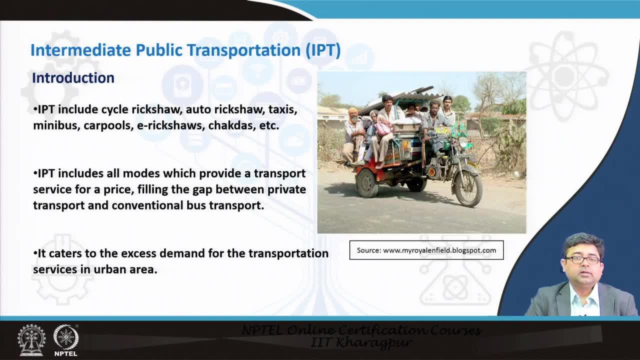 system, For example, cycle rickshaw, auto rickshaw, taxis, minibus carpools, even the new e-rickshaws that are currently available in many cities. IPT usually caters to the excess demand for transportation services in the urban area. So sometimes what happens? 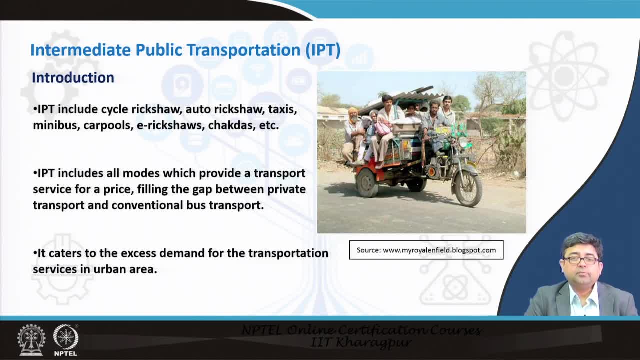 is, the demand is such that it is not being met by the public transportation system that is there. But at the same time it is not financially viable to increase the access or improve the public transportation system. right, So it is not yet viable to have another metro line in your city. But 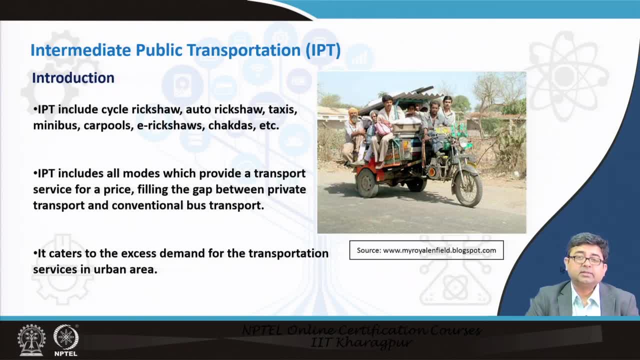 you can already say that the demands for the existing metro line has been surpassed. So during such times IPT also becomes very, very important, where they are now almost supplementing your, your existing public transportation system in your city. So that has also been noticed. 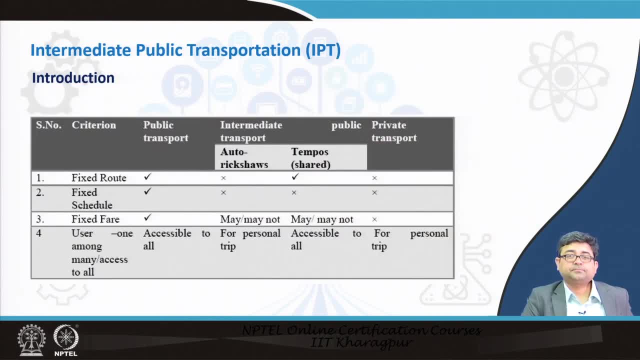 in many cases, especially in India. If you compare them to public transport systems, they are usually more flexible, both route wise and schedule wise, So you can hire a taxi to go anywhere anytime. They do not run on any fixed schedules. they can run on your schedule. Usually their fares are a little. 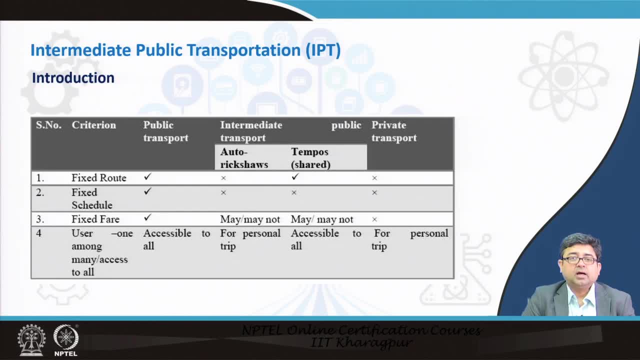 bit higher than public transportation systems which almost always have some fixed fares based on distance or so on and so forth. So many cases you get the flexibility with your IPT but you might have to pay higher fare and sometimes you may also see that public 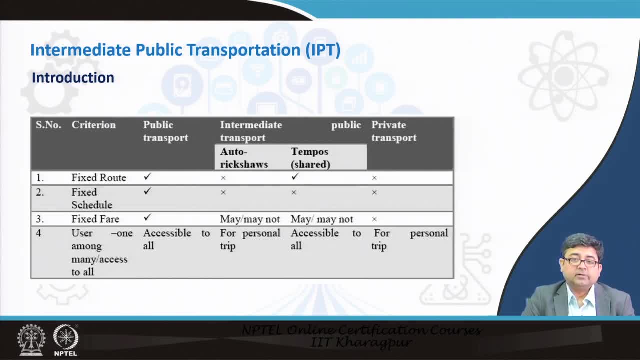 transportation systems are more flexible, So that has also been noticed. in many cases, public transportation systems, or IPT, is acting very similar to a public transportation system, especially when IPT also allows a vehicle to be shared by multiple people. So that is when they resemble a public transportation system. 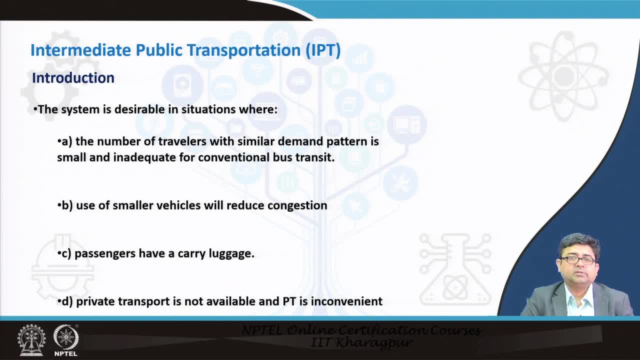 The system IPT is desirable under several circumstances. but if you can look at it from a very policy perspective or a very high level perspective, you can say that when the number of travelers with similar demand pattern is small and inadequate for conventional bus transit- So when the demand is very less- what happens is a bus transport system becomes. 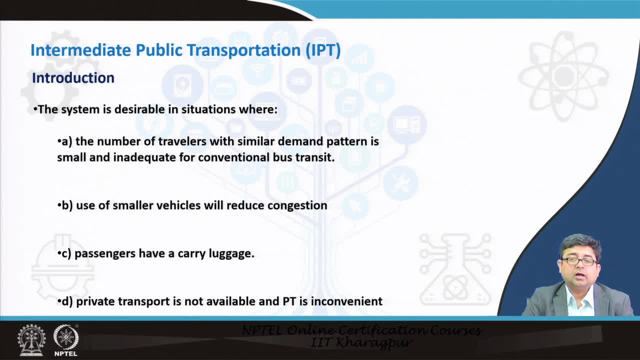 financially not viable. We have already looked at how bus transport revenues are collected, how they can be generated through transit marketing. So, despite all of those strategies, even if then you cannot financially or your bus transport system is not financially viable, in those cases IPT becomes the only alternative. 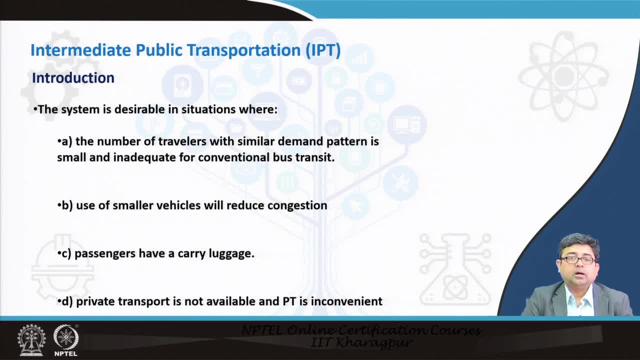 for your city. Alternately, the use of smaller vehicles will reduce congestion as well. So if your streets are very narrow, especially in smaller towns where you do not have wider roads, and if you have buses- or at least the new generation buses- that are much wider and longer and require a large turning radius, that may not be very. 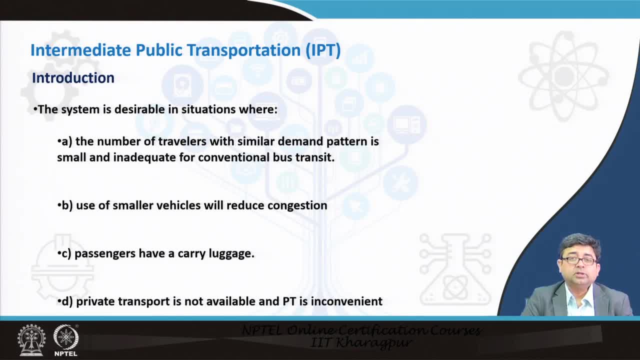 feasible for your city or for your small town. So in these cases also you will see that the smaller vehicles or the smaller IPT vehicles becomes very popular. Usually they always cater to people If you are carrying some kind of a luggage, so that becomes your almost private taxi. 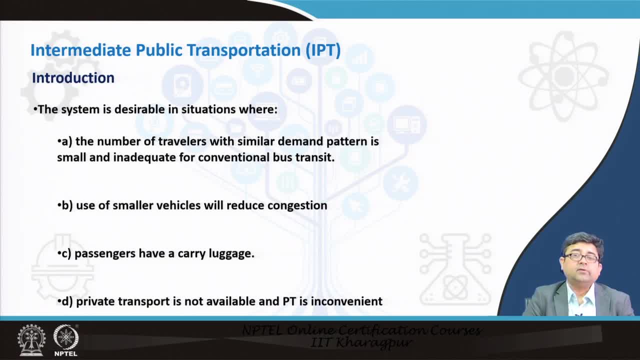 any IPT, any auto, rickshaw and taxi allows you to have a space to put your luggage, and hence people always prefer them while they are going to their destination. And if the private transport is not available and PT is inconvenient, so if you do not own any, 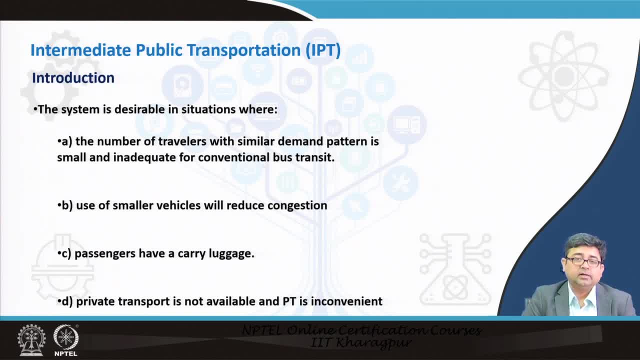 vehicle or you are not in a position to own position to own vehicle and public transport is too few buses per hour, or there is no metro or the metro is too far away from your house. in such cases, public IPT also becomes very, very important or starts paying a major role in the public transportation system of your. 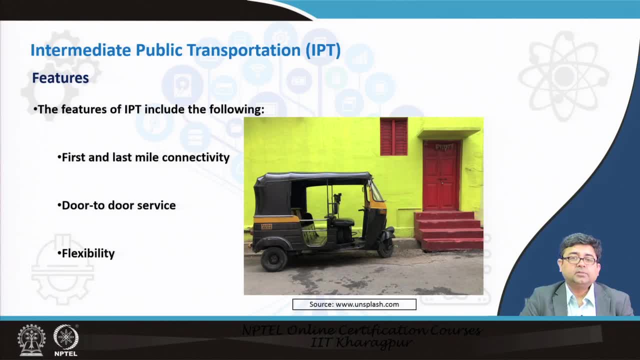 city. It does provide the first mile and the last mile connectivity, and hence they are becoming very, very popular. The auto rickshaws will take you from your door to the destination door, whereas fixed route public transportation systems- your buses- will not, do not provide that last mile. 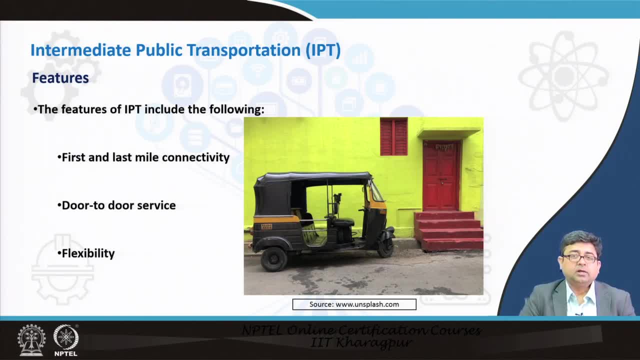 connectivity. So IPT as a genre started becoming very, very popular Because of this facility that it provides. it provides door to door facility. it is flexible, so you can avail it anytime you want to avail it, so that allows you to not own a vehicle. 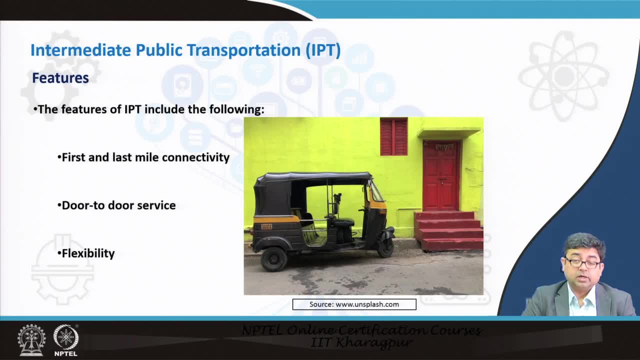 as well. So your cost of owning vehicle goes down as well, but your flexibility remains. so, with, the biggest advantage of owning a vehicle is the flexibility that you get. Now, if the same amount of flexibility is being provided to you by the intermediate public transport system, or the IPT, then you are. 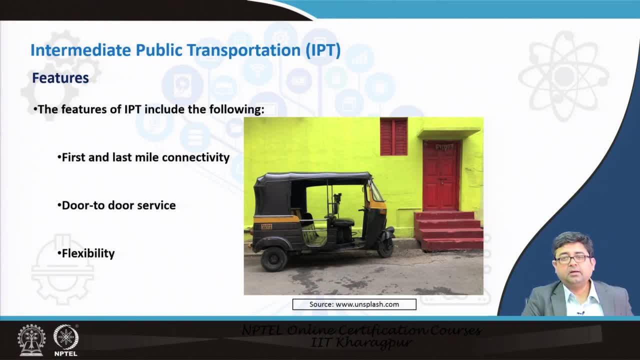 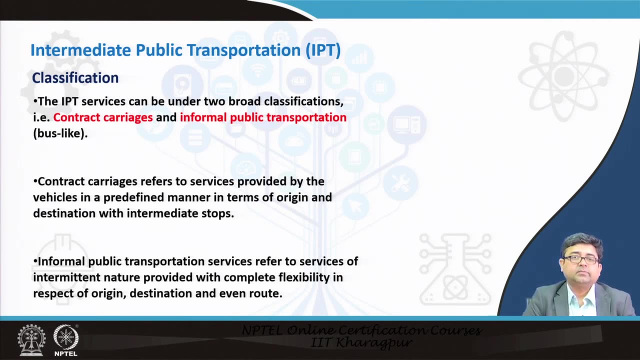 saving on the cost of, or the capital cost of, buying a private vehicle yourself. So those are some of the advantages of IPT system. There are two broad classifications of IPT system, if we can look at it in that way. one are contract carriages. 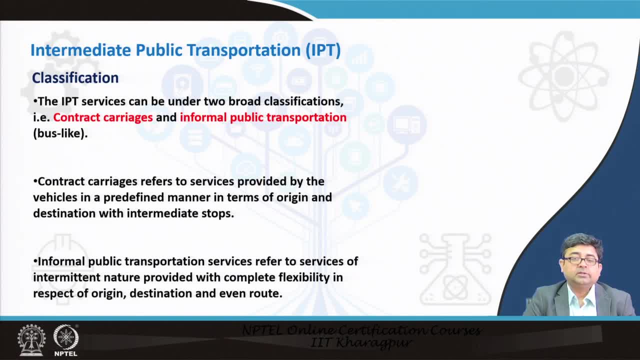 and one are more informal public transportation, which look like, look, feel like a bus system, but really is not a bus system or is not a part of your entire city network. They are only in pockets and certain parts of the cities or they are contract carriages. 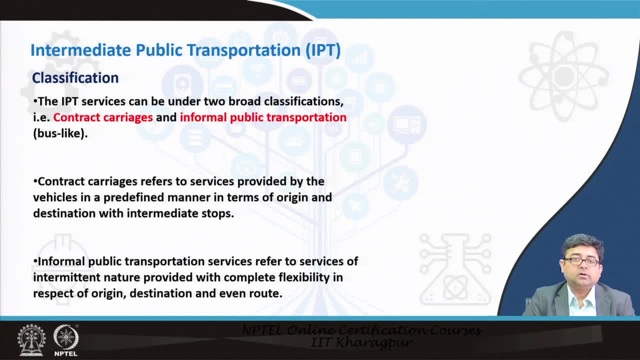 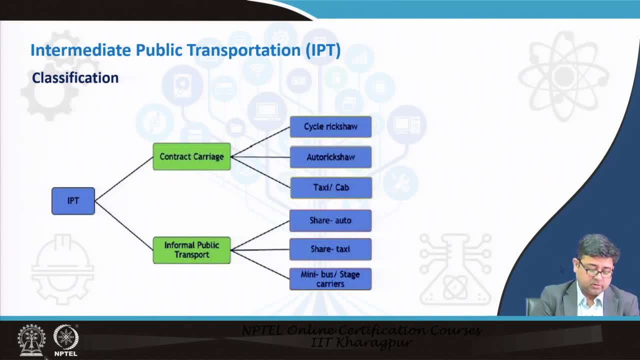 like your rickshaws and auto rickshaws or cycle rickshaws, So this gives you an idea of what we are talking about. So, for example, if you are talking about contract carriages, your cycle rickshaws and 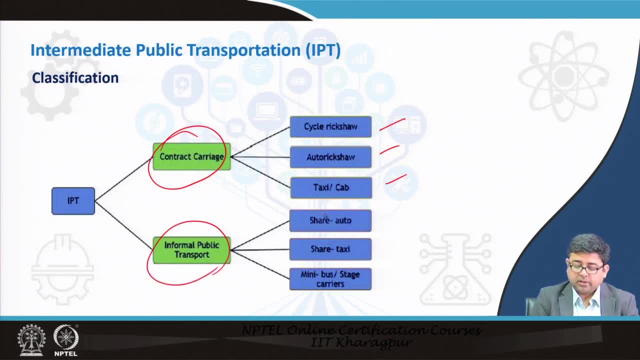 cabs, whereas if you are talking about informal public transport, wherever you are sharing something, it becomes a. it becomes something of a informal public transport. right In many, in many cities, you would see that you can. you can share autos. there are shared. 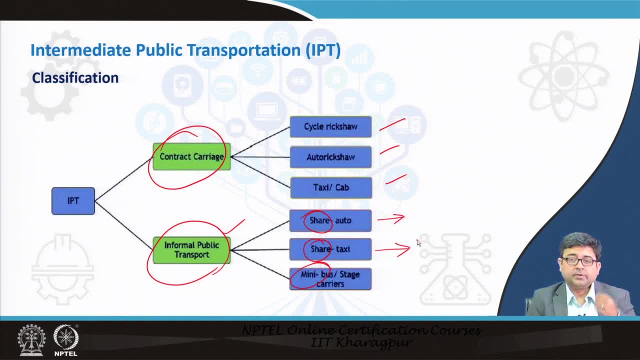 taxis, Even the new. So, Ola Obers, you can, you can, you can ride with others to save cost. So that is, that is, those kind of category, those kind of vehicles, those kind of services come under the informal public transport category of IPT, otherwise you have your for hire. 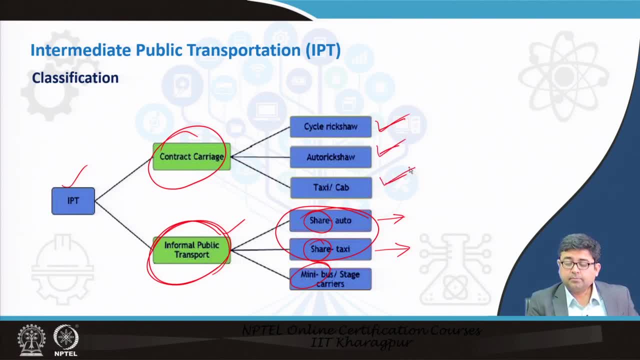 So these are mostly you can use for as a private vehicle, right? You can just hire a cycle rickshaw for wherever you want to go, So you are not sharing it with anybody. You can hire an auto rickshaw. 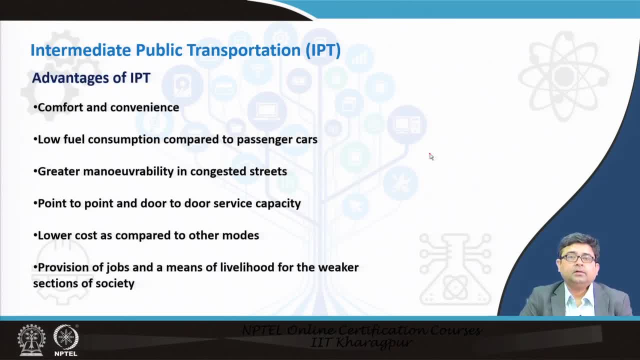 You can hire a taxi or a cab. So the advantages of IPT are are are many fold. You you can have the comfort and the convenience that was otherwise being offered by your own private vehicle. Now you can get it through the use of a IPT. low fuel consumption when compared to passenger. 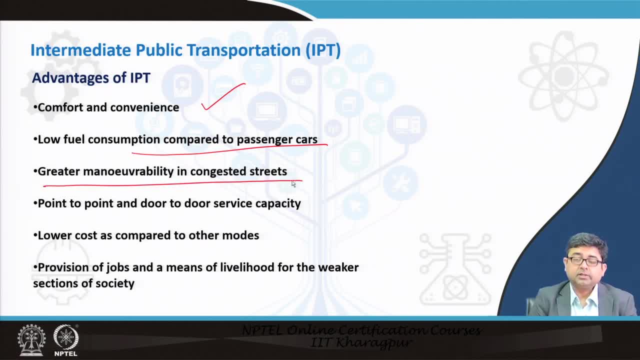 cars Greater maneuverability, Especially in congestion, Especially in congested streets. So we will see how that that sometimes can be can have a negative connotation as well. But you must be very well aware of how auto rickshaws especially can maneuver through. 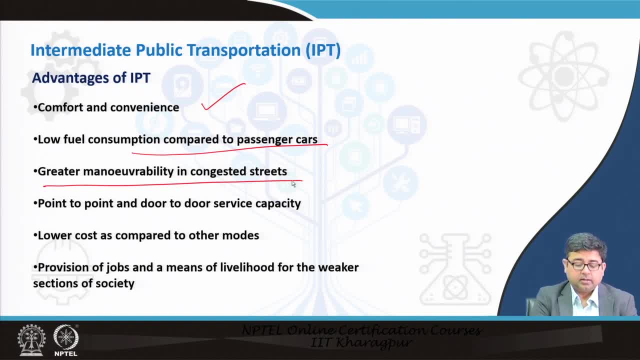 the traffic in congested streets obvious. Of course they provide the door to door service and the cost is if, especially if you are sharing, the public transport vehicle is usually much lesser, even when, or is lesser or even comparable to your much larger city wide public transportation system. 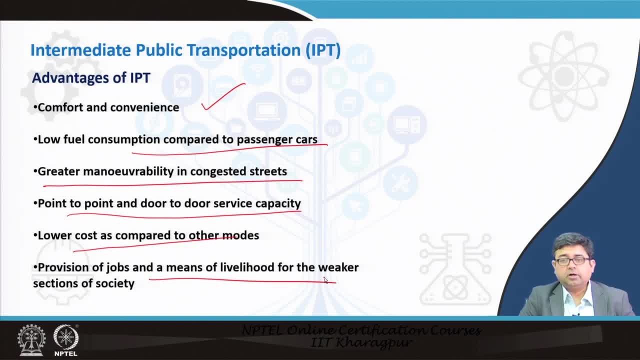 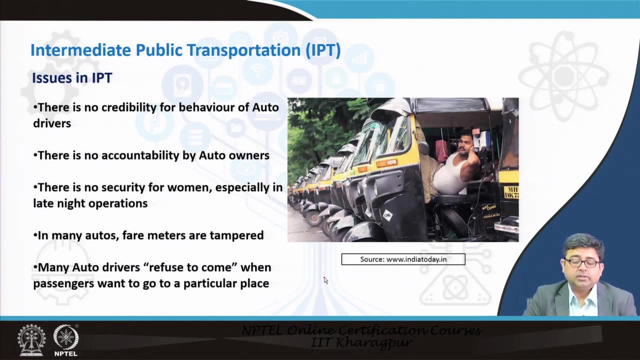 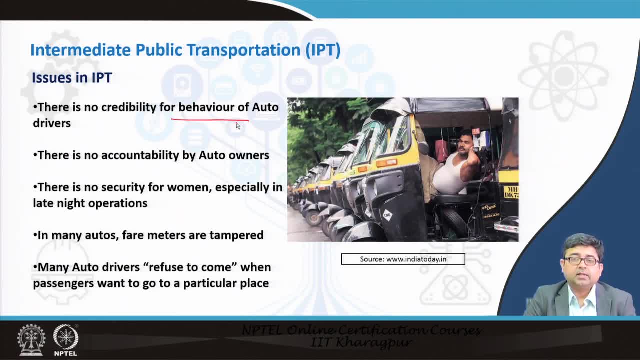 when they reject trips. that has become a major issue in many, in many cities across India. They would not want to go to a certain area to drive. They would not want to go to a certain area to drop you off because they know that the trip. they may not get a person for the trip back from there. 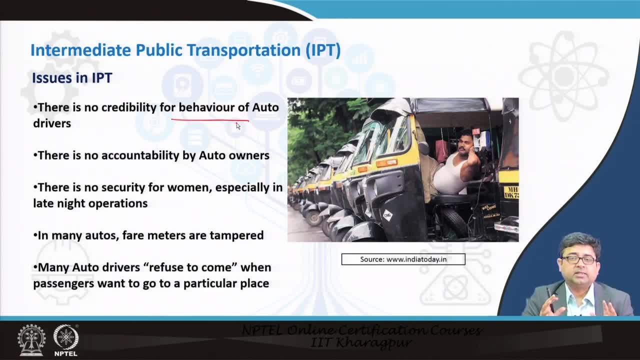 So the demand, if your city or if your destination is in a area which has lower demand for for them, they, they would reject, they would reject that trip, and then that leaves you in a in a dilemma, or that leaves you in a situation where You are left with no alternative but to use your public, use your own private transport. 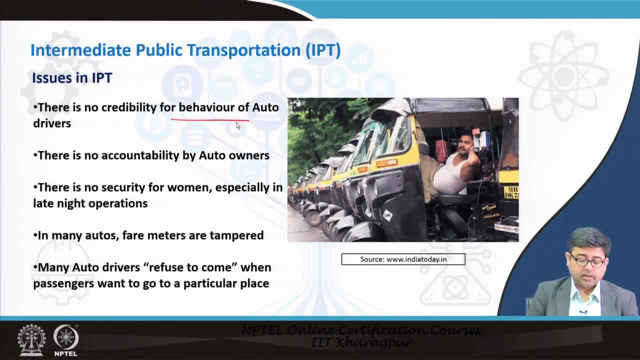 use your own car or two wheeler. there is no accountability. many times you see poorly maintained auto rickshaws. sometimes when the auto rickshaws are being shared, you see that there are too many people sitting in an auto rickshaw. there are efforts being made to improve accountability. 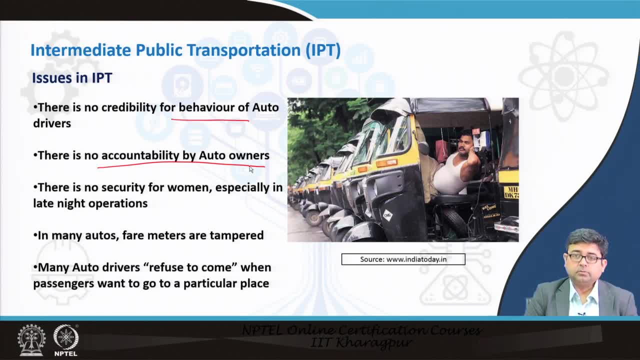 Technology, but that is lacking in many, many cities across the country. night operations and security for women are an issue, and in many autos, what you would notice is that the fares are, or the fare meters are, tampered with. So how do you have better enforcement of fares while using auto rickshaws is something 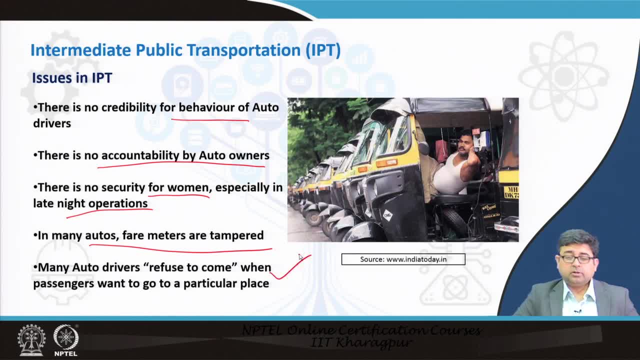 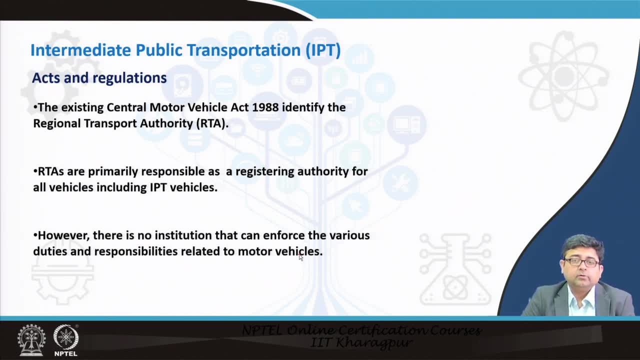 that is being looked into and we have already talked about the refusal part. When we look at the issues, we then try to look at what are the acts and regulations that can help solve these issues, but the existing Central Motor Vehicle Act of 1998. 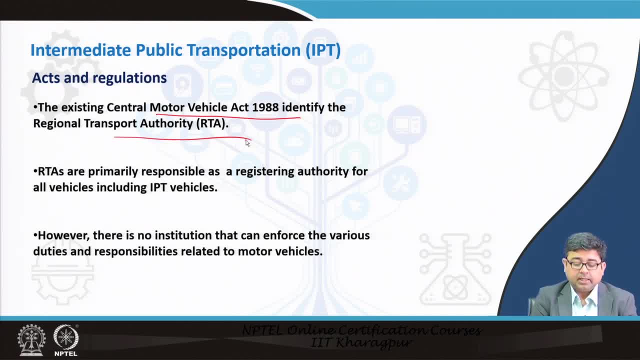 requires any regional transport authority. They are responsible for registering all the IPT vehicles. However, they cannot enforce the various duties and responsibilities related to motor vehicles. So they can only register them, but the behavior and the operations of these IPT vehicles are not being enforced by many of these acts. They do not detail. 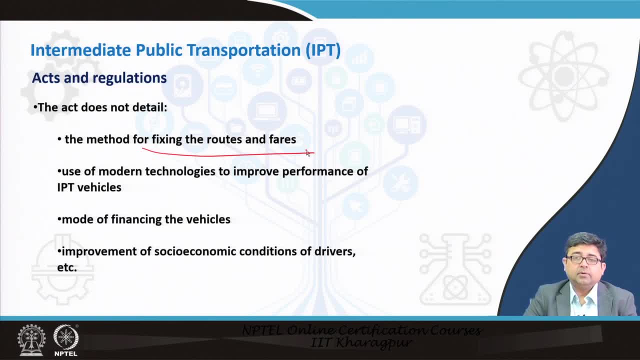 the method of fix, fixing routes and fares- Remember this is one of the major issues with hailing taxis or auto rickshaws- is because of the different fares that they can ask for while rejecting a trip or even rejecting the use of a meter. Many times you have seen that or we have experienced. 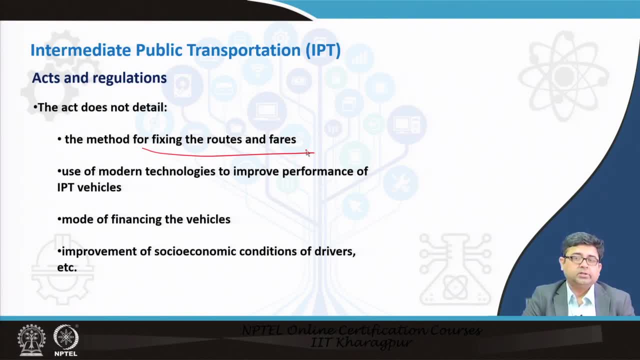 that they would not go by meter and they would just charge a flat fare. So there is no way or no mechanism in place that can regulate all of those things. There should be acts that also incorporate the modern technologies of tracking where you are. So 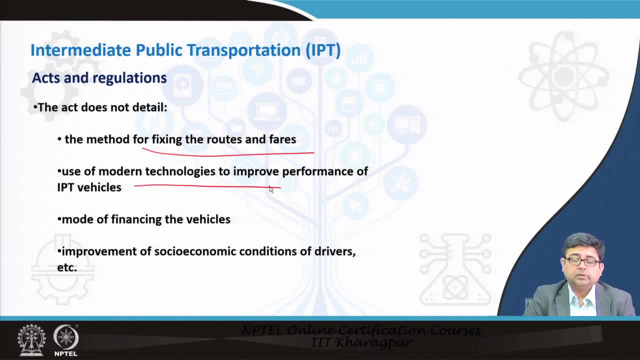 now in many cities, even auto rickshaws are coming into the fold of the transport network companies, TNCs or the Ola Ubers. There is an overall competition of over autos or Ola autos, where now you can actually know beforehand what is it going to cost and also 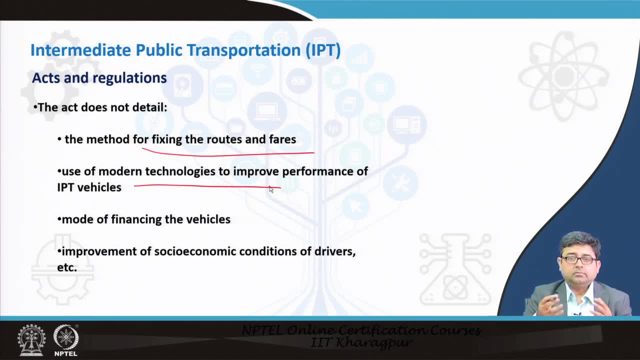 where the auto rickshaws is and you can, from the security point of view, you can inform your friends and family where you are. There is no. the act does not cover how to finance those vehicles and also how to improve the, obviously, how to improve the socio-economic. 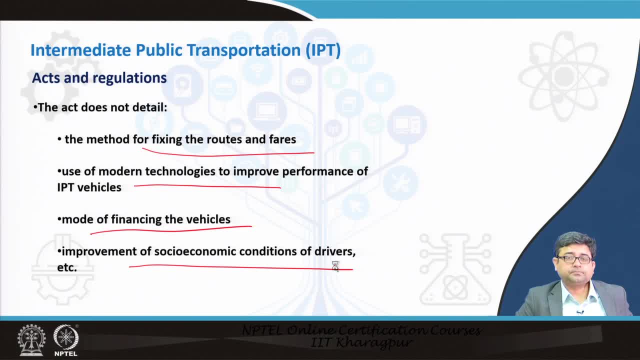 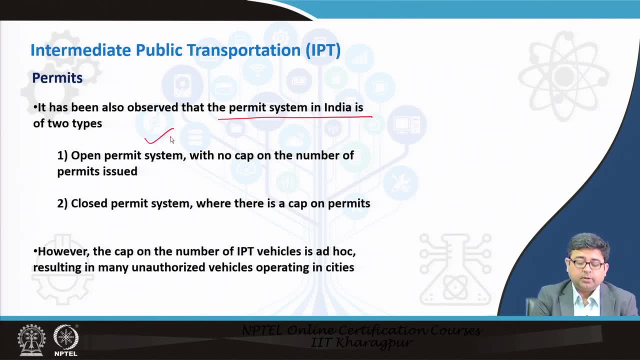 conditions of the drivers covers is also not being looked at. It has been also observed that the permit system in India usually is of open permit system or a closed permit system, where there is a cap on the number of permits, but when it comes to IPT vehicles, the permitting is very ad hoc and there is no limitation of 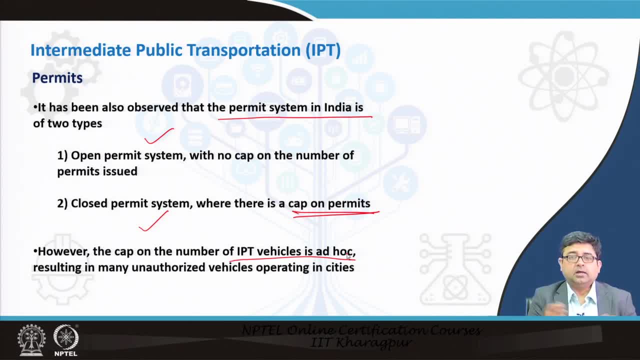 the number of registered IPT vehicles in any of the cities, and that in many times causes a conflict with the existing public transportation system as well, where now the ridership of public transportation systems in some of the cities are declining, whereas the usage of IPT systems is increasing. 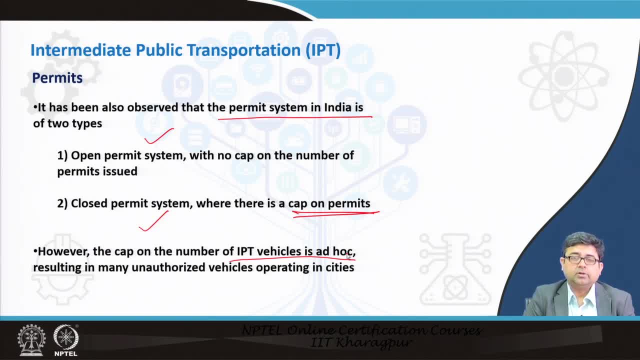 So many urban transports are not being used in India. It is not being used. So many urban transports are not being used in India. So many urban transports are not being used in India. transport planners are worried with that situation. now saying that, whether IPT system should. 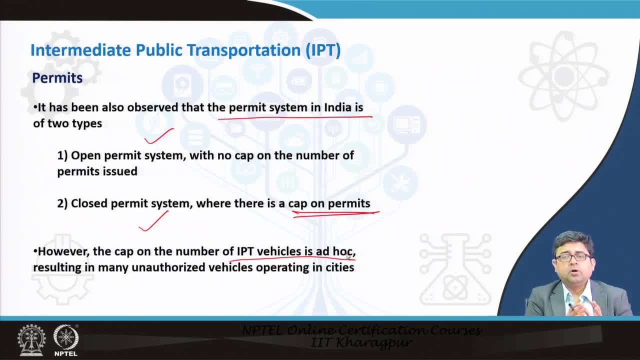 only act as feeders to the public transportation system or whether they should be a parallel public transportation system in themselves. So if they are a parallel public transportation system, then they are now competing against the existing bus network or metro network, whereas if they are feeding to it, then they 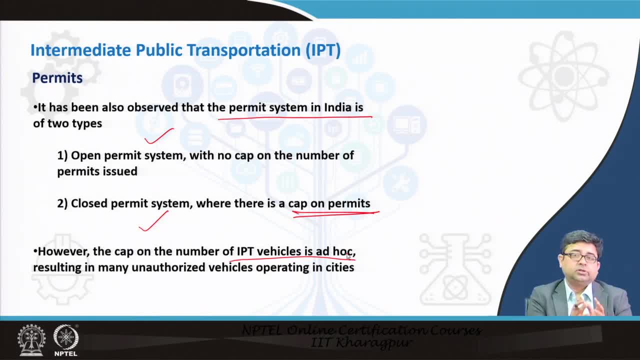 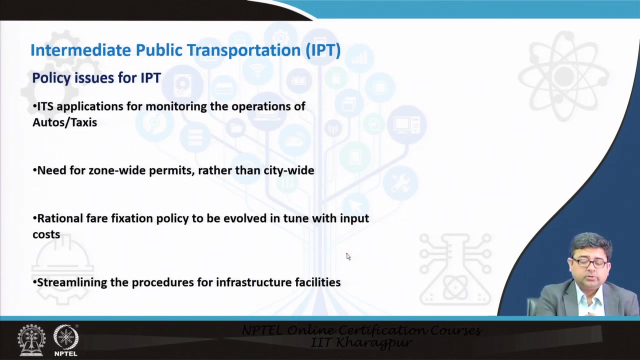 are acting as a acting for a different purpose, So should they be complementing the larger public transportation system or should they be supplementing and competing with them is something that many urban cities or many urban locations are already dealing with. When you look at some of the policy issues for IPT, like we already mentioned, there are 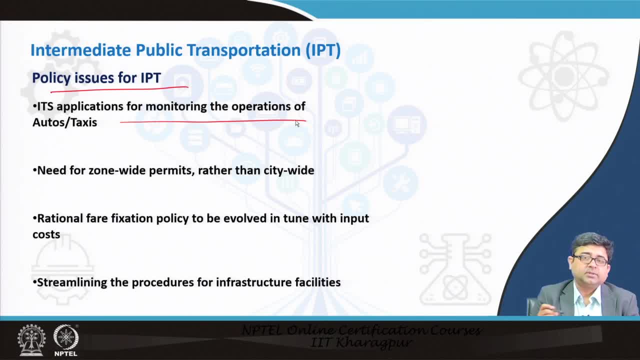 several ITS applications now That will allow you to track, especially if they are registered or if they are part of any of the transport network companies such as Ola or Uber, So that allows you better security. There is a need for zone wide permits rather than city wide. 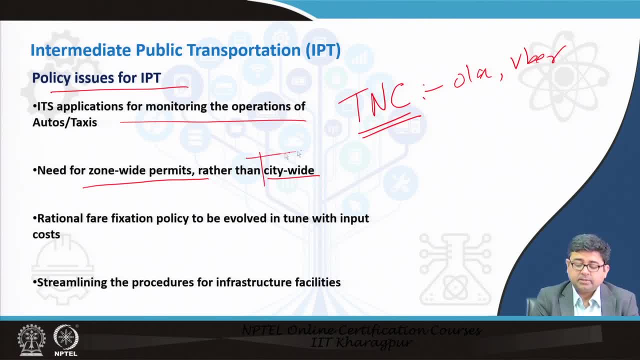 Certain IPTs. if they have city wide permits, then they become more like a public transportation system itself. So now you can take it from one part of the city to the other. So they are almost Supplementing the public transportation system rather than feeding it to it. 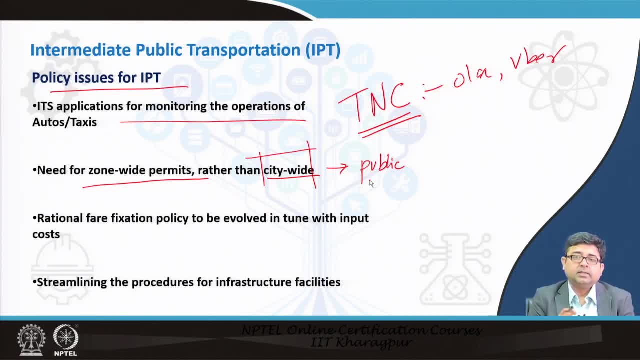 But whether if they are only regional permits are given or zonal permits are given, then they are more likely to be feeding to the larger public transportation system. There should be rational fare fixation policy. It cannot be that in night hours they can charge whatever they want to or when they. 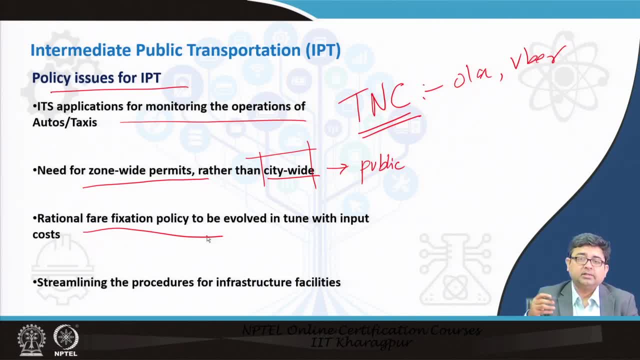 are travelling to a destination which has lower demand, they can charge higher fees. So there has to be, You have to have certain kind of fare fixation policy. that is a bigger debate. that is also going on when you talk about your Ola or Uber systems, when they ask for a surcharge or when 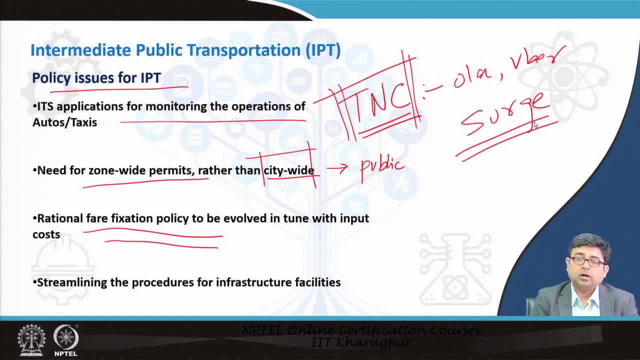 there is surge pricing. How do you control or how do you put a cap on the maximum amount that can be charged? that is also being debated under this umbrella of fare fixation policy. and there has to be procedures. There have to be procedures for streamline, procedures for providing particular infrastructure. 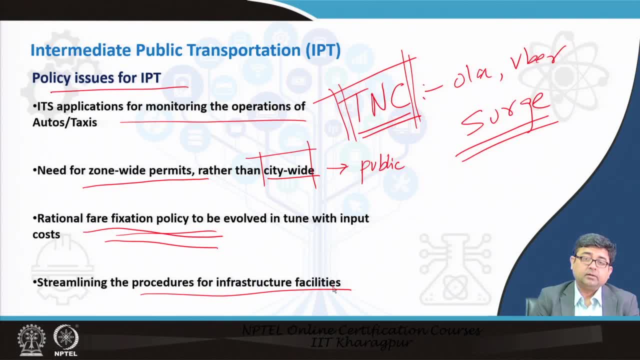 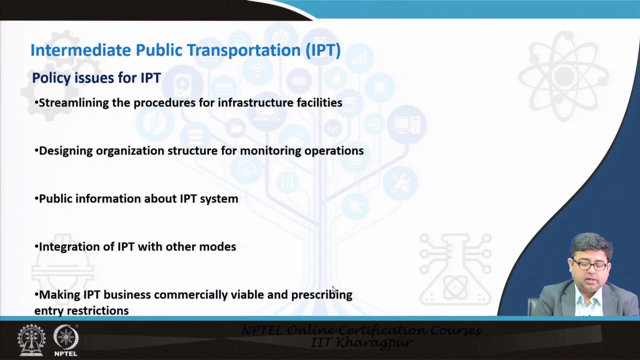 facilities for them as well. Especially, having proper auto stands or rickshaw stands near larger public transportation hubs is very essential in order to allow the traffic to flow in an unimpeded way and not allowing people to hail. So if they are acting as feeder systems to the larger public transportation systems, 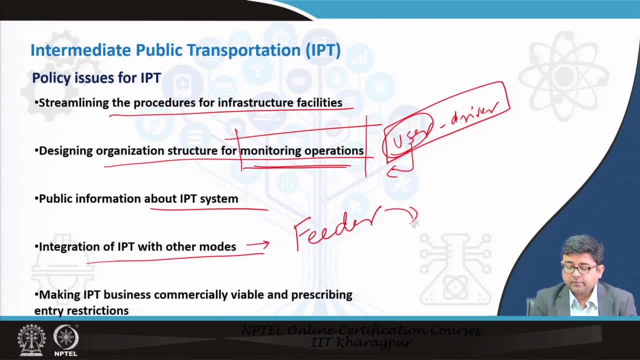 they have to be integrated with them. So when you get off from a metro station, you have to make sure that there are sufficient number of auto rickshaws at the stand. You can then have a seamless multimodal journey rather than you get off a metro station and 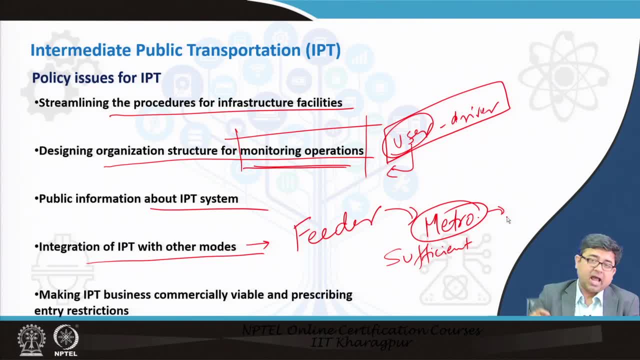 then you have to wait for 10-20 minutes that adds to the your travel time, and then many times you are reluctant to use the public transportation system. So IPT has to be integrated with the existing public transportation systems and of course they have to be commercially viable.